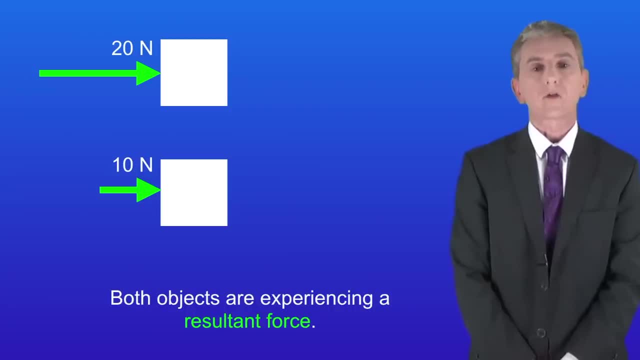 here two objects with equal masses. Both objects are experiencing a resultant force. the top object's experiencing a resultant force of 20 Newtons to the right and the bottom object is experiencing resultant force of 10 Newtons to the right. Now, as we said before the acceleration of 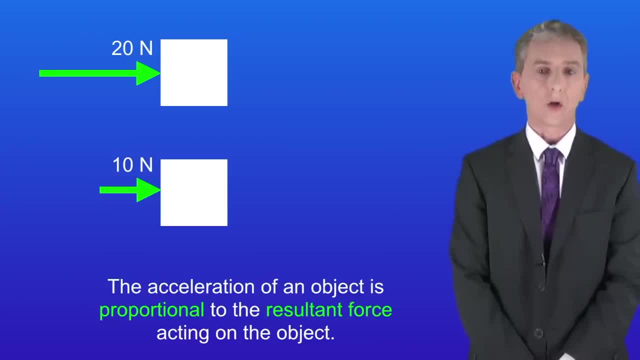 an object is proportional to the resultant force acting on the object. What this means is that if we've got a greater force, then we have a greater acceleration. So this means that the top object will experience twice the acceleration of the bottom object. Okay, this shows another two objects. 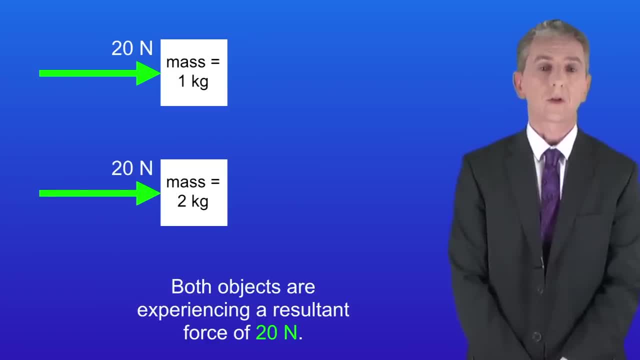 and both objects are experiencing a resultant force of 20 Newtons. The top object has a mass of one kilogram and the bottom object has a mass of two kilograms. As we saw before, the acceleration is inversely proportional to the mass of the object. In other words, if the mass is larger, 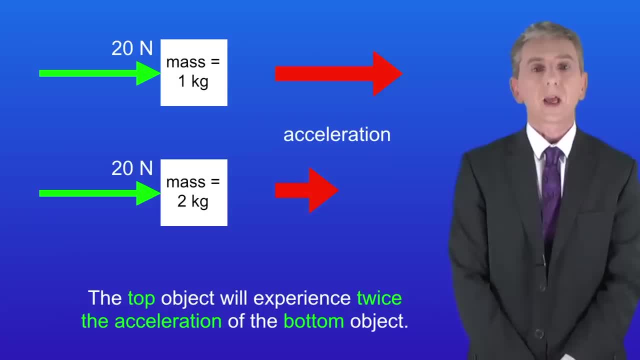 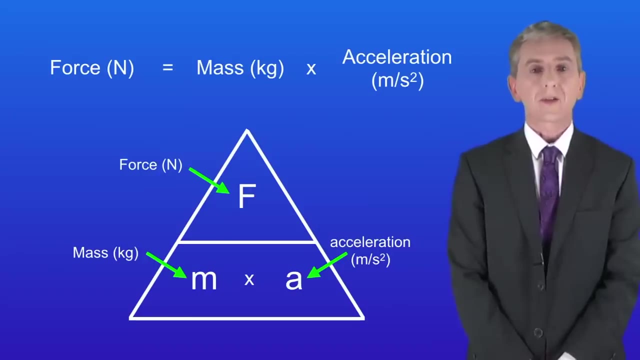 then the acceleration will be smaller. So once again, the top object will experience twice the acceleration of the bottom object. Now we can use this to calculate the force needed to accelerate an object. We use this equation: The force in Newtons equals the mass in kilograms multiplied. 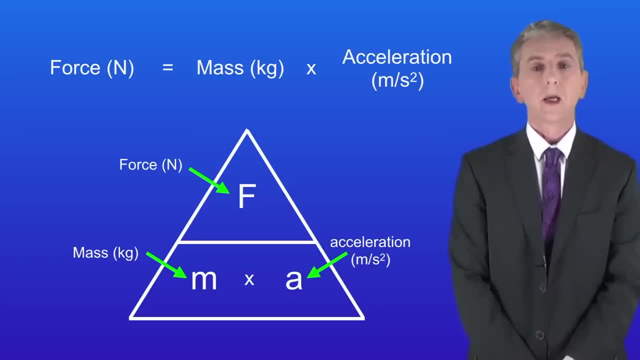 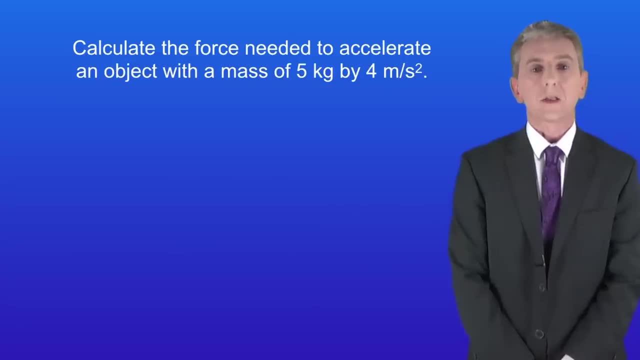 by the acceleration in meters per second squared, And you are not given this equation in the exam, so you need to learn it. Here's a question for you: Calculate the force needed to accelerate an object with a mass of five kilograms by four meters per second squared. So 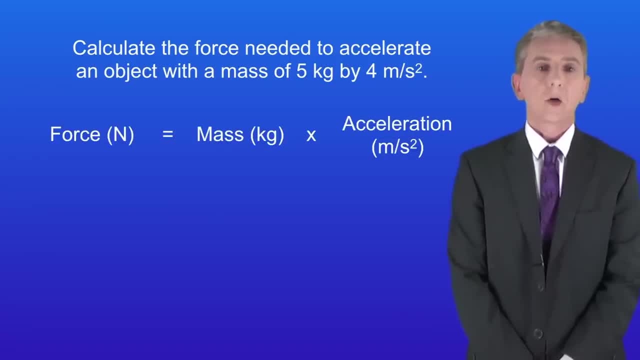 pause the video now and try this yourself. Okay, the force equals the mass multiplied by the acceleration. The mass is five kilograms and the acceleration is four meters per second squared. Putting these into the equation gives us a force required of 20 Newtons. 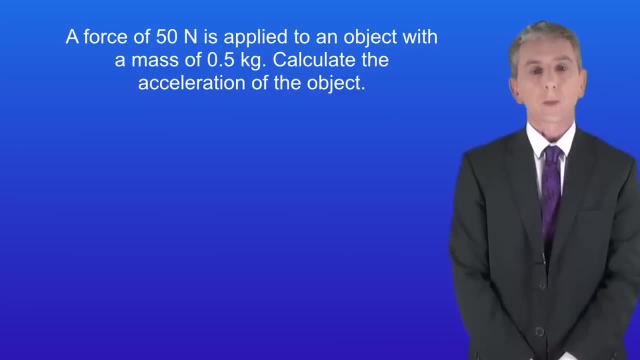 Here's another question for you. A force of 50 Newtons is applied to an object with a mass of 0.5 kilograms. Calculate the acceleration of the object. So again, pause the video and try this yourself. Okay, in this case we need to calculate the acceleration. Looking at the triangle, we can. 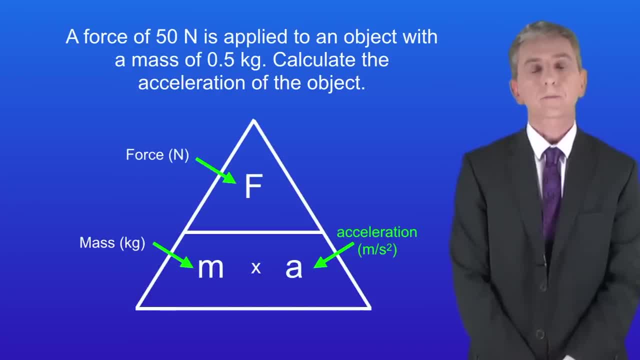 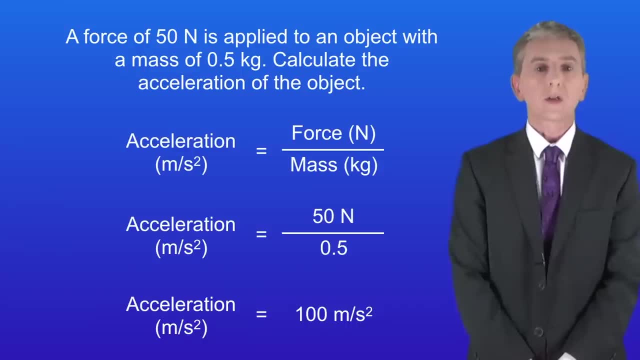 see that the acceleration is the force divided by the mass. In this case, the force is 50 Newtons and the mass is 0.5 kilograms. Putting these into the equation gives us an acceleration of 100 meters per second, squared. Okay. now in the exam you could be asked to estimate the speed.